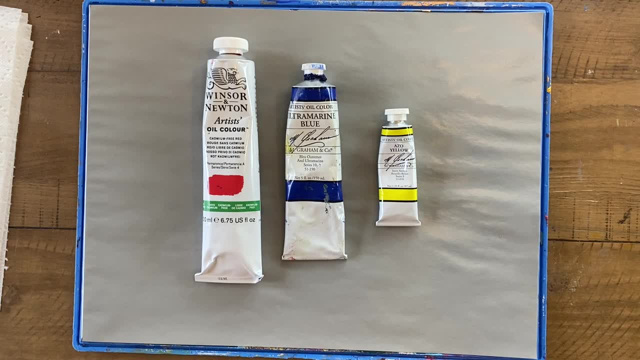 the primary colors, But it turns out we have some reason to doubt both of those things. In the art world, primary colors are something of a controversial subject. Can you actually get every color out of red, blue and yellow, And are there other candidates? 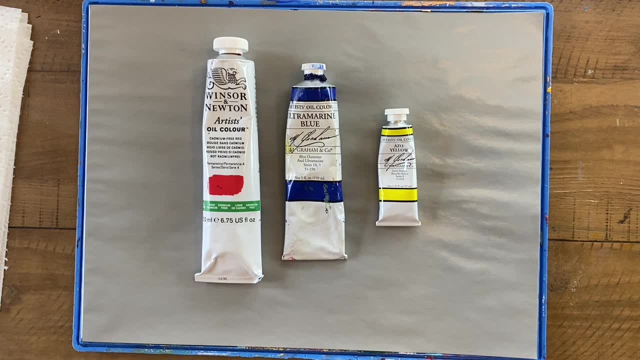 out there for the primary colors. Is it true that you can't mix the color red? It turns out that not everyone views red, blue and yellow as the primary colors, And they have other candidates that they say are the true primary colors. 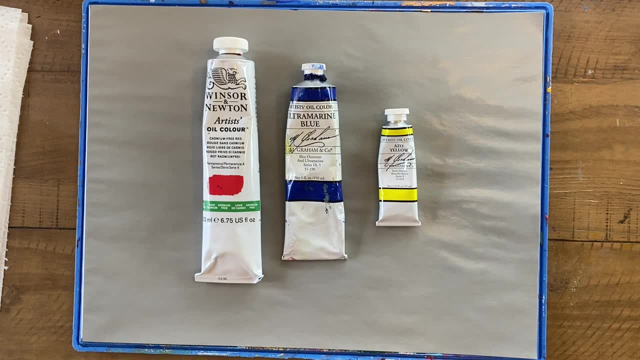 This video is a primary colors showdown, where I pit primary colors against each other to find out what are the true primary colors. Or are they even like the Highlander, where there can be only one? I'm going to be taking four different sets of primary colors and mixing a color wheel. 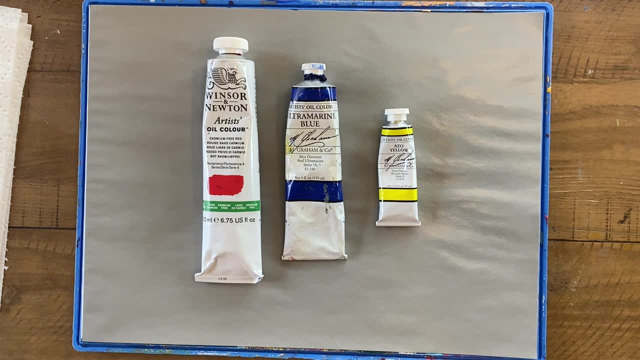 out of each one With the color wheel that I mix. I'm also going to take each mixed color and stick it on a digital color wheel to see how my range of possible colors for that primary stacks up against the full range of colors that actually exist. So let's get color mixing. We're going to start off with the 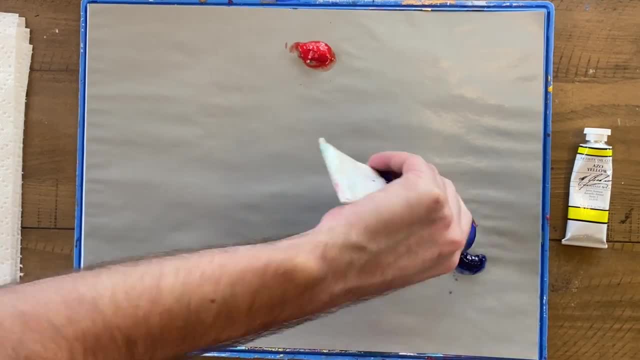 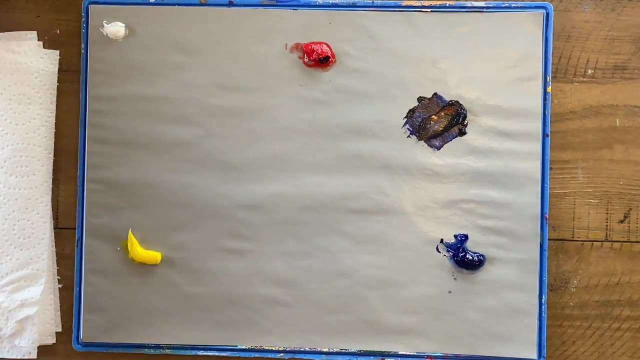 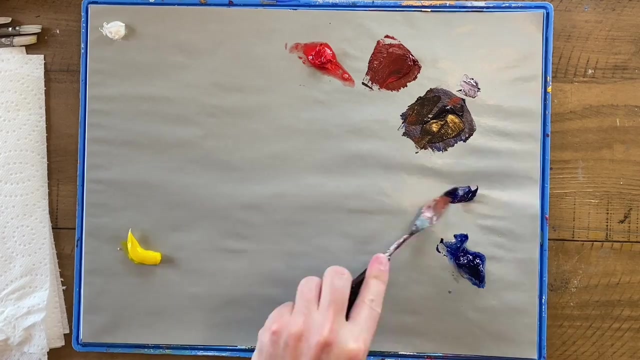 traditional three primary colors: red, blue and yellow. Now, the results that you'll get out of color mixing are highly dependent on which- red, blue and yellow you choose. So I kind of just have to make a judgment decision on which colors I want, But these are the ones that I like to use. 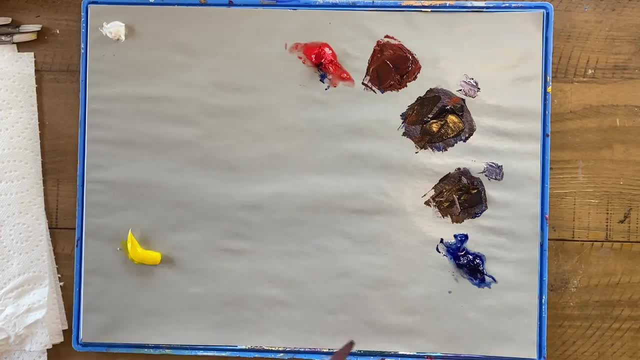 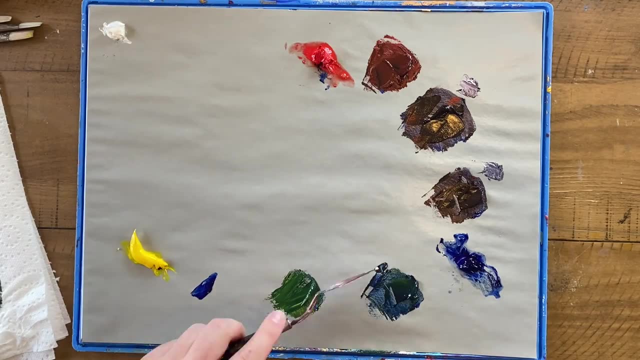 in my painting. So if you happen to use, say, a cadmium yellow instead of this, your color wheel is going to look a little bit different than mine. One of the things that you'll already notice as I'm making this color wheel is, while I can get red, blue and yellow, I'm also going to get red blue. 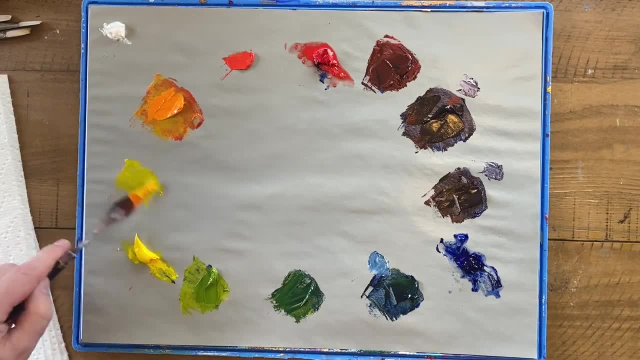 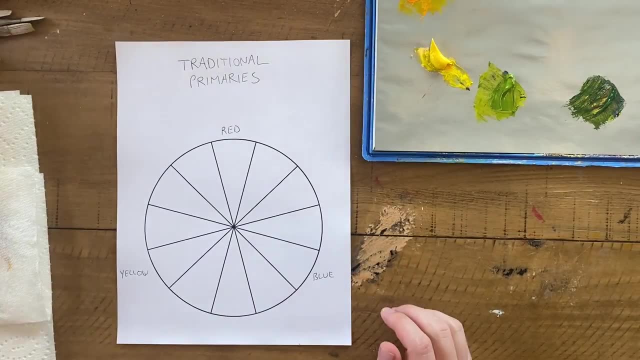 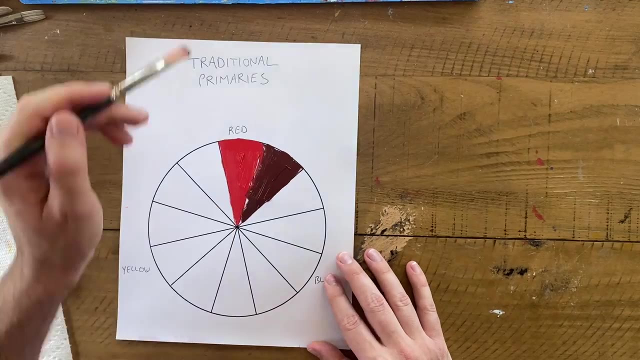 and orange. So if I get very vibrant reds and oranges, I actually get a pretty dull looking purple, And this shows us something about color mixing in general. Color mixing is subtractive. What that means is you lose saturation when you mix two colors together, Using our purple color. 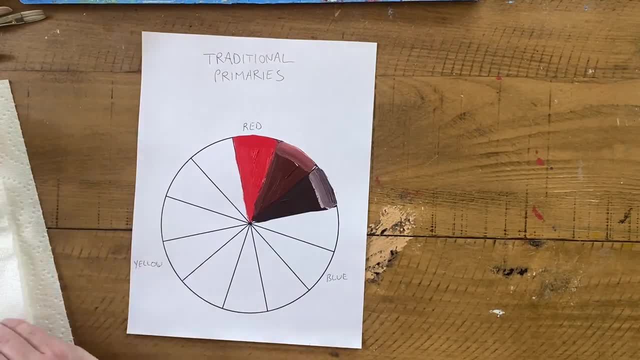 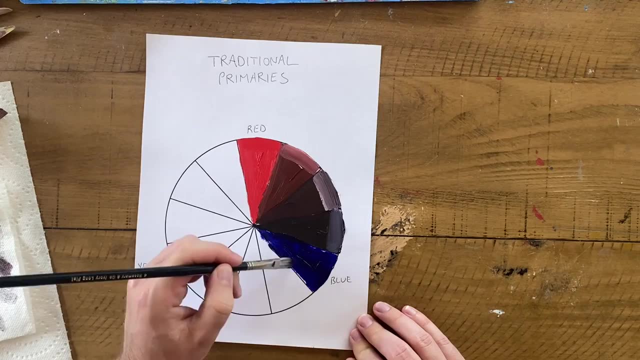 as an example here. I'll never be able to mix a purple that is as saturated as a purple that I get straight from the color wheel. So I'm going to use a red, blue and orange And I'm going to from the tube. So we're already seeing that the first thing I learned about primary colors as a 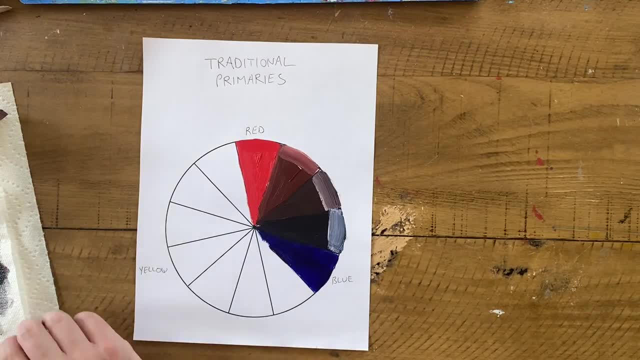 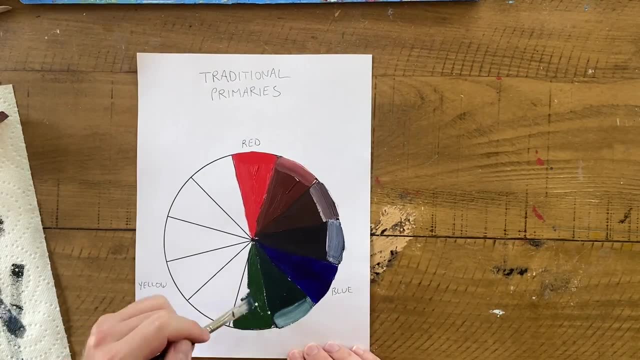 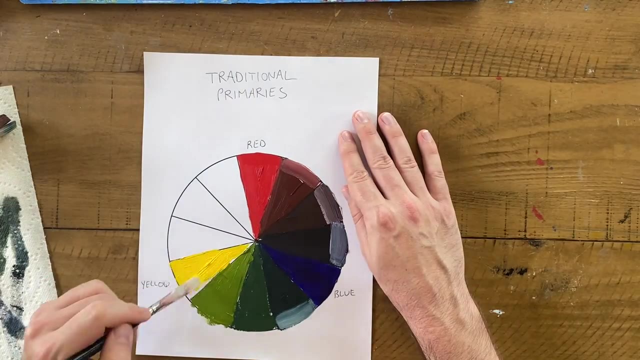 kid is not true. I can't technically mix every single color out of these primary colors. Our three primaries give us a range on the color wheel, not the whole thing. So it's not true to say you can mix every color in existence from primary colors. It's true to say I can mix every hue. 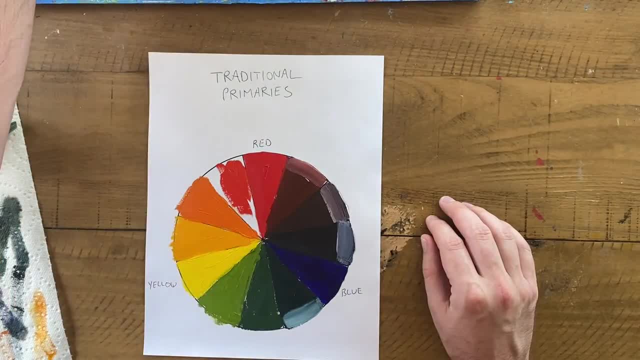 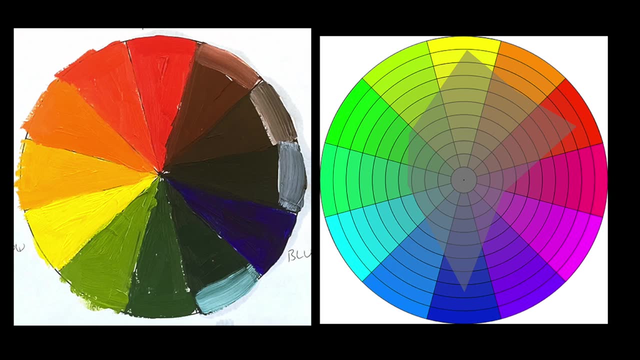 I can get some kind of a purple, but I can't mix every color. And now we'll take this color wheel and we'll map each color onto my digital color wheel And this color wheel may look a little bit different to you. This is called the. 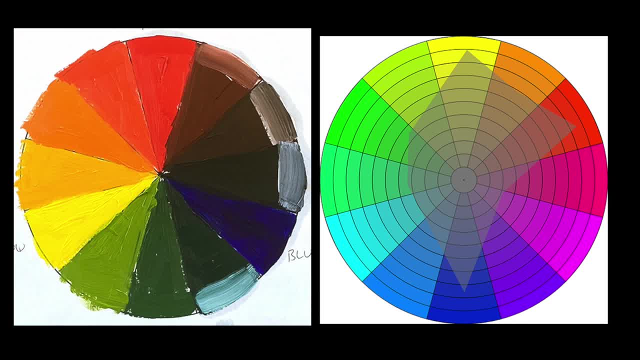 Yerby color wheel And the benefit this one has is that it spaces out the actual distribution of the color spectrum a little bit more accurately than our traditional color wheel. So out of my red, blue, yellow primary colors, here are the colors I can actually attain. I can get really vivid, warm. 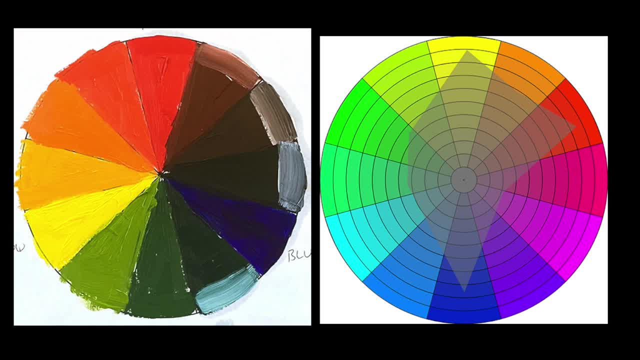 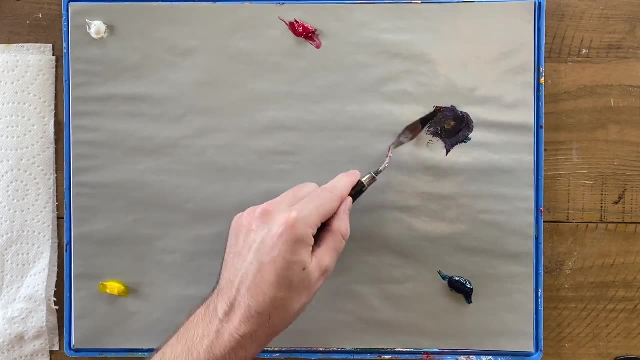 colors: bright blues and even- okay- greens, but my range of purples is low. I'd also probably be wanting more greens if I were painting a landscape. Okay, now we're going to do a really fun one. The hardcore color geeks out there will be aware of what I call the printer's primaries: cyan, magenta. 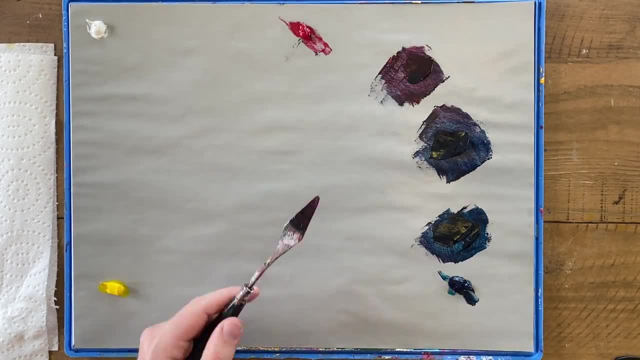 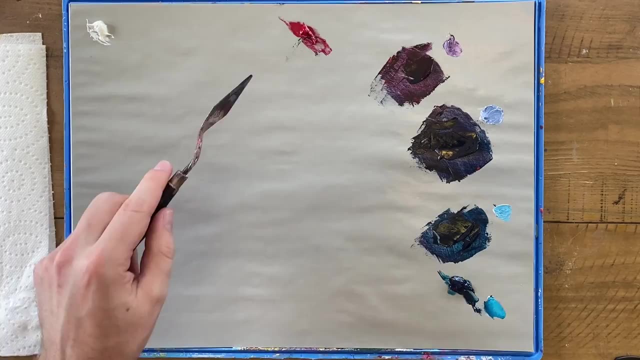 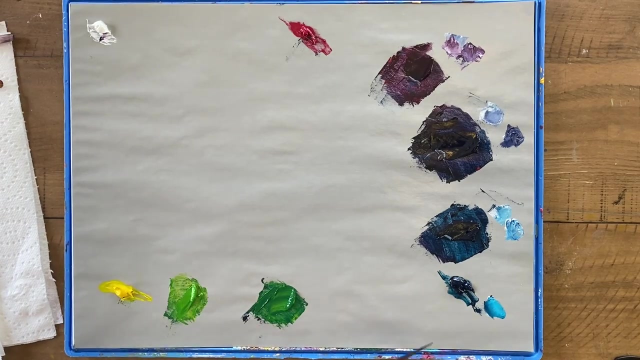 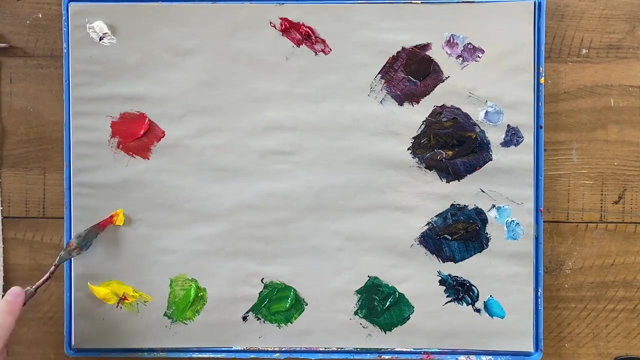 and yellow. These are the primary colors in your color printer. You may have seen C-M-Y-K on your printer ink before, and that's what they're talking about: Cyan, magenta, yellow, and then K stands for black, And so for my printer's primaries I'm going to be using quinacridone rose for my magenta, phthalo turquoise for my cyan and azoyellow for my yellow. 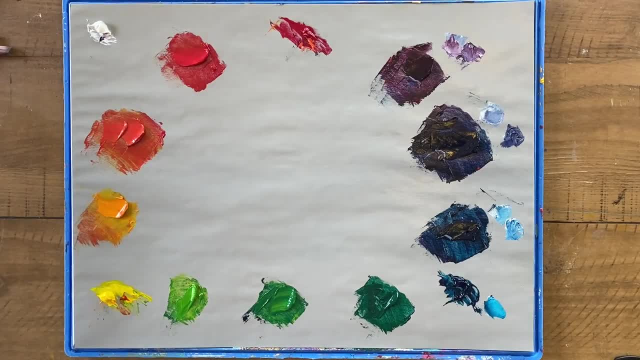 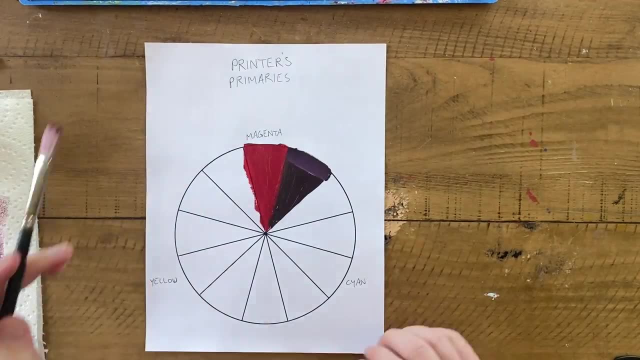 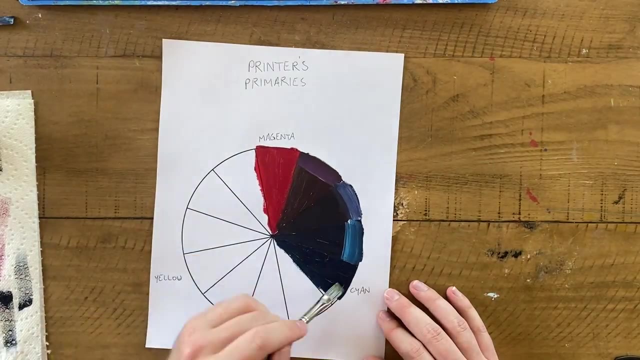 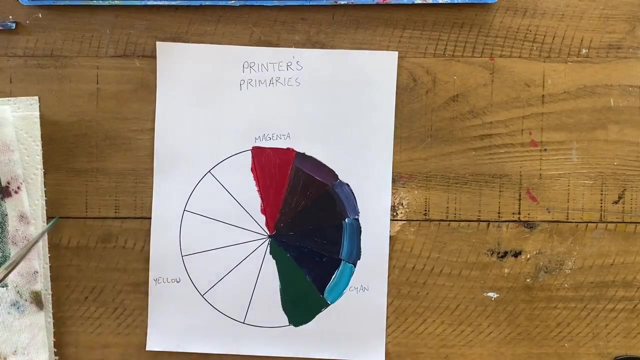 The existence of these primary colors raises a serious question. I've been told that primaries are colors that can't be mixed. So is that true? Can I mix magenta and yellow together and somehow get red? Can I mix cyan and yellow and get blue? Let's find out. Well, it turns out, you can mix red and. 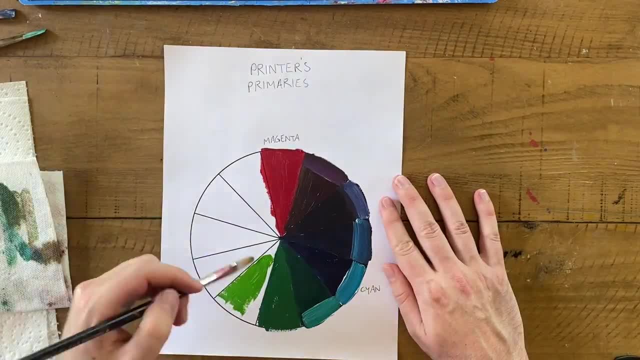 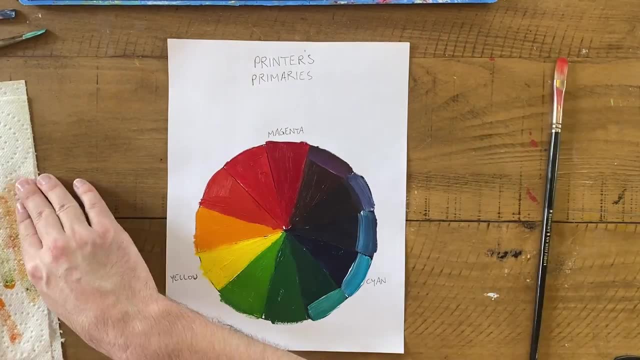 blue. Honestly, this was mind-blowing to me. the first time I saw it I was like, oh my god, I can't remember the first time I did it. So after this, I guess cyan, magenta and yellow are the real primaries, right? 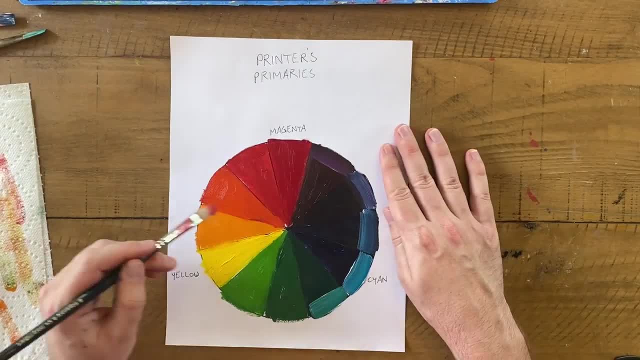 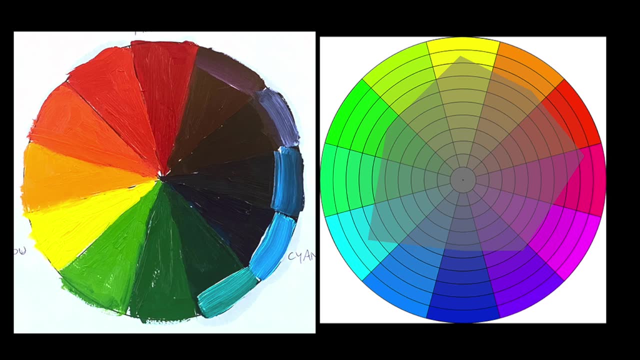 Well, not so fast. Let's map our mixed color range onto our color wheel. We see here that these primaries share the same limitation as our red, blue, yellow primaries: We can access only portions of the color wheel. In fact, you can see that, compared to the first primaries we have, 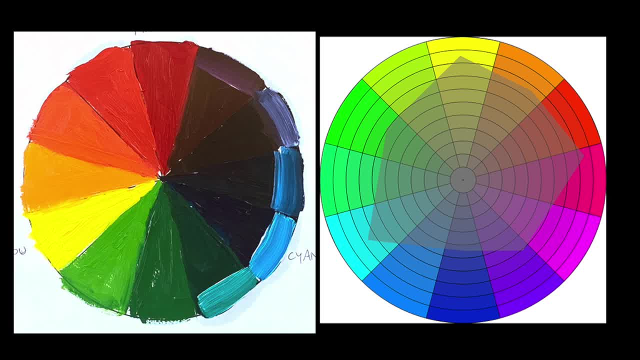 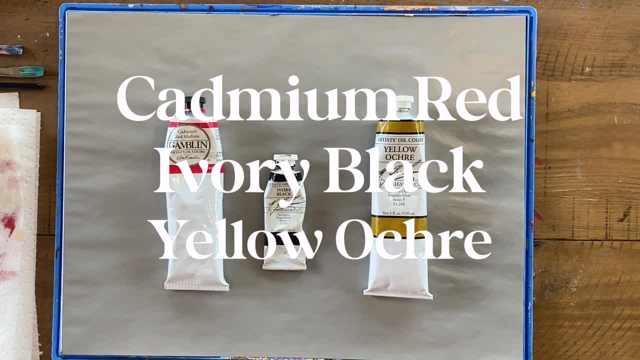 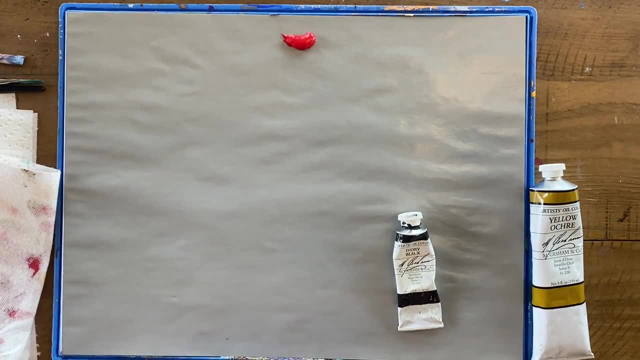 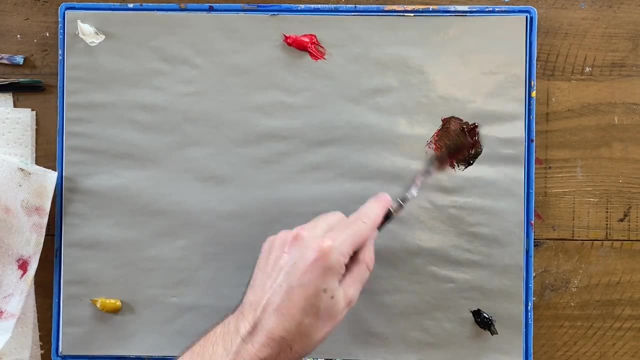 So for our third set of primaries, we're going to be doing something totally different. We're going to be using the color red, black and a really dull yellow. So you may ask yourself, why would I ever choose to limit myself by taking three primary colors? 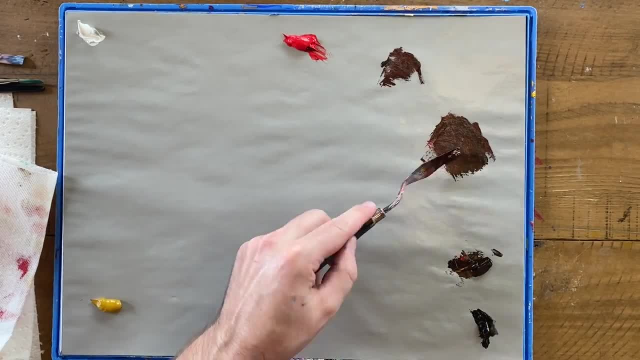 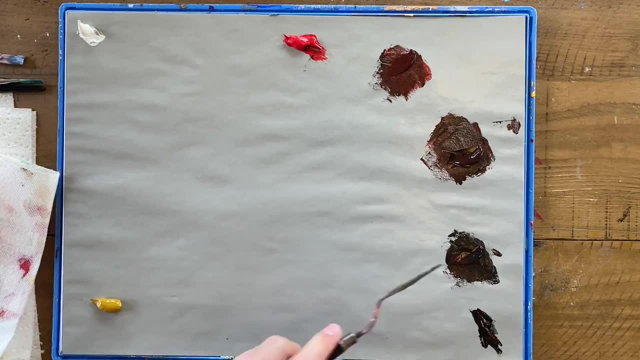 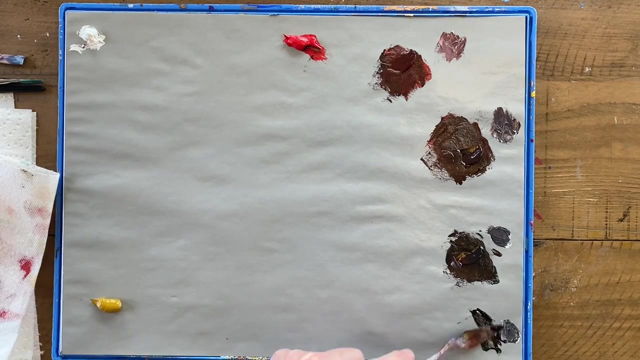 that are already pretty neutral even before I mix anything together. One of the reasons is, if you choose a set of primary colors that already have limitations built into them, the colors that you end up mixing together will have a uniformity and a coherency that is really beautiful. 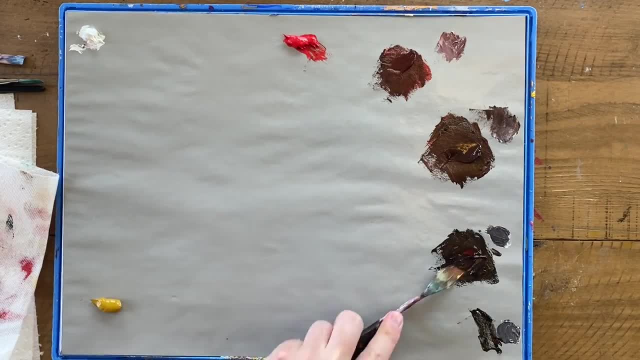 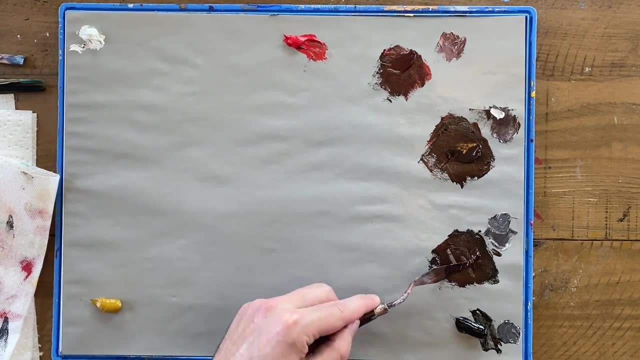 When every color is just a little bit closer to every other color, they all hang together in this really lovely way. Another reason you may want to limit your primary colors is you could choose primary colors that best suit the subject that you want to paint. 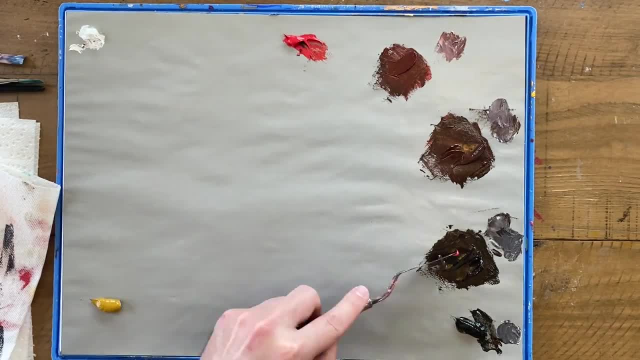 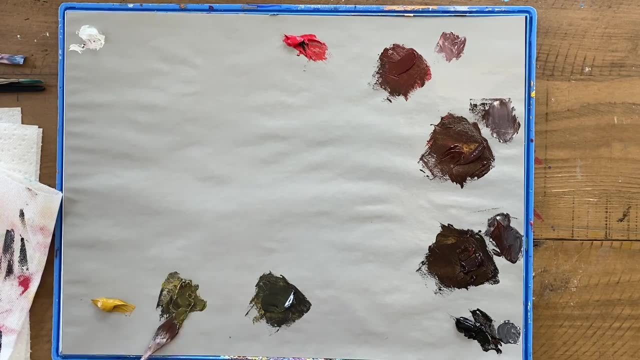 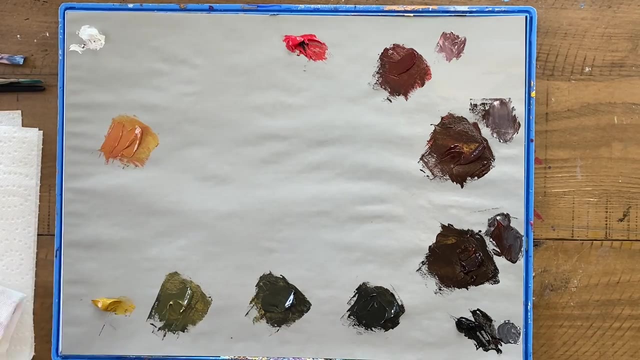 This palette of colors here is actually very popular among portrait painters. It's something called the Zorn palette, which was created by a painter named Anders Zorn, And one of the benefits of this palette is it lends itself to getting really great flesh tones really easily. 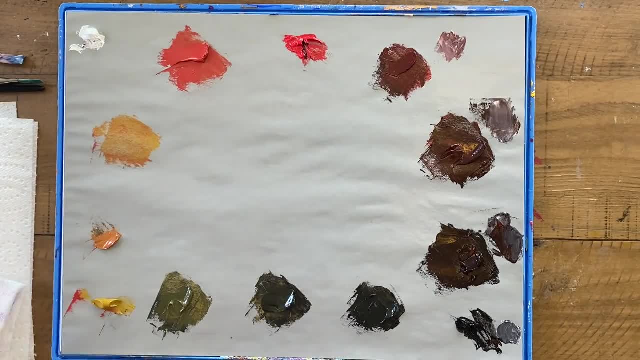 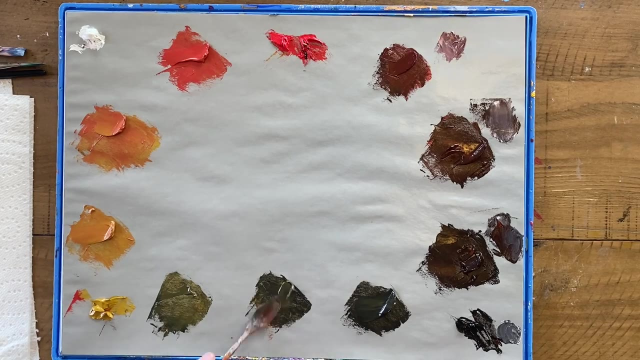 So I talked about how limiting your primaries lends itself to every color in your painting that you're painting, And I want to talk a little bit more about what I mean by that. When you have access to absolutely any color you want, I think you run the risk of your 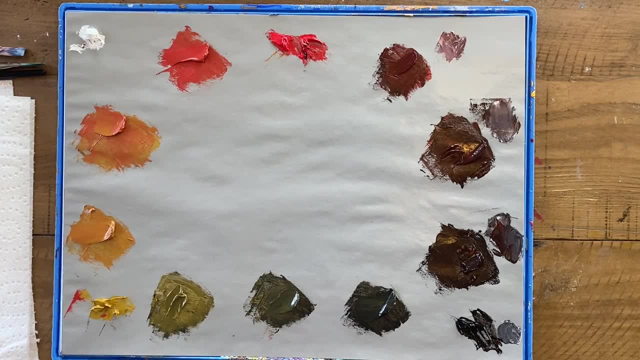 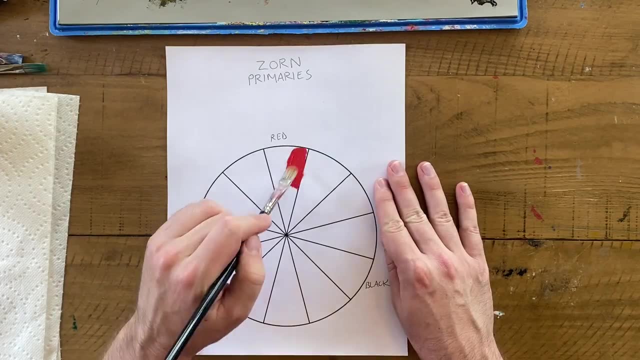 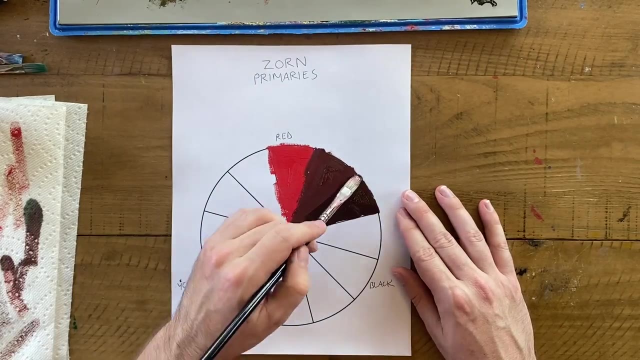 paintings looking garish and unrealistic. Think of some landscape painting that has overly green grass and overly blue sky. It kind of looks like something a child might have made. It takes a lot of subtlety and discipline to tone your painting. You want to tone your colors down to make them work together. 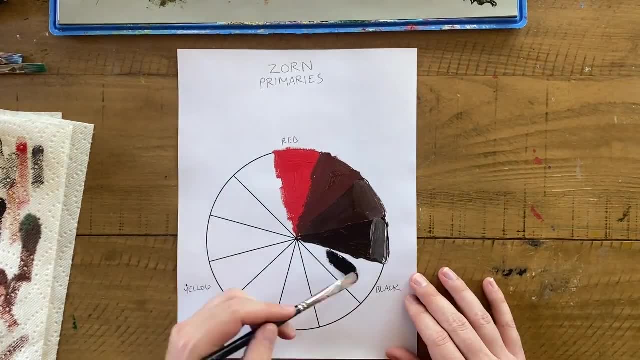 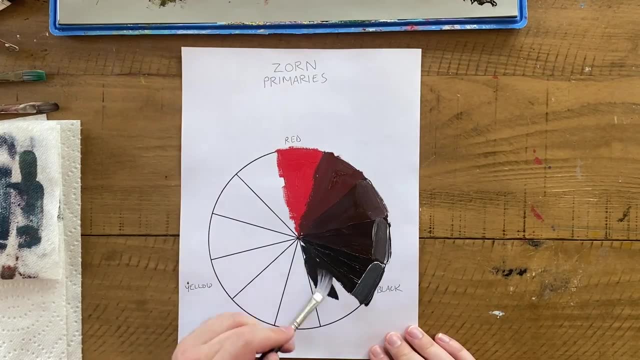 And a limited palette takes care of this, naturally. Now, of course, there's nothing wrong with a painting looking unrealistic, and for colors to quote, unquote, not hang together. It all depends on what you're going for, And there are no rules in art. 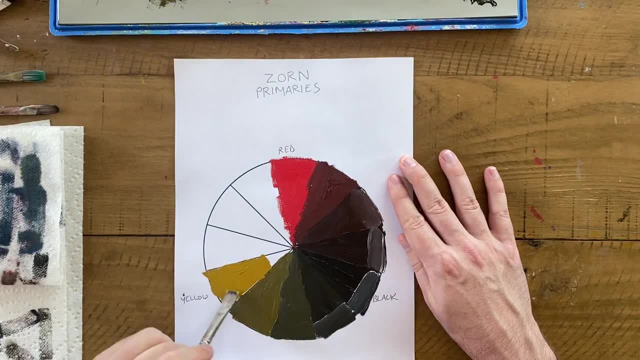 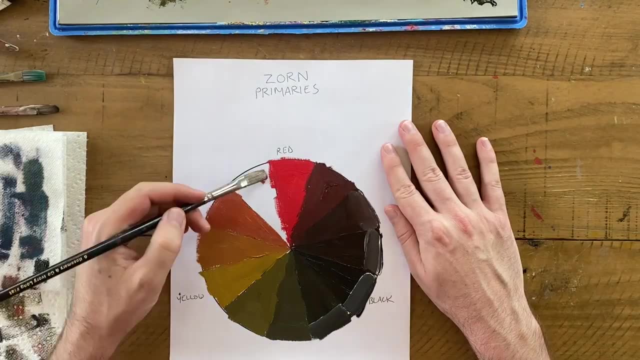 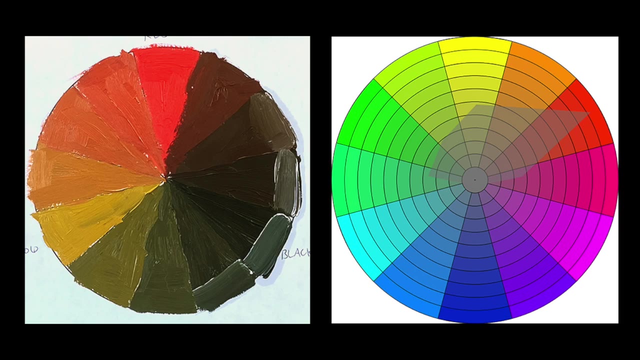 But if you're dissatisfied with the realism of the colors that you're creating, using a limited palette can really make your job a lot easier. So let's see the range of colors that we can get out of the Zorn palette. All right, so here's our Zorn primary color wheel. 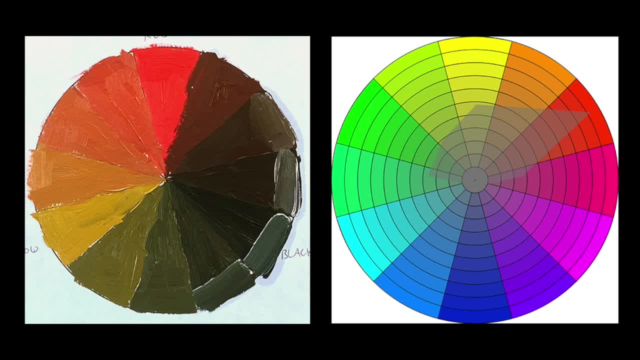 And talk about a limited palette. The only vivid color that we have to work with is the red, And the yellow is looking pretty vivid now compared to everything else around it. You'll see that between red and black is basically just a long variety of different browns. 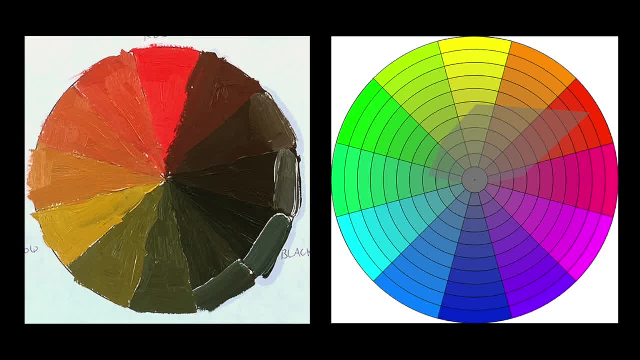 But if you're going to use a limited palette, you're going to want to make sure that you're using a limited palette. But an interesting thing happens when you use this palette. If you look at a painting that's done with the Zorn primaries, you'll see that the color 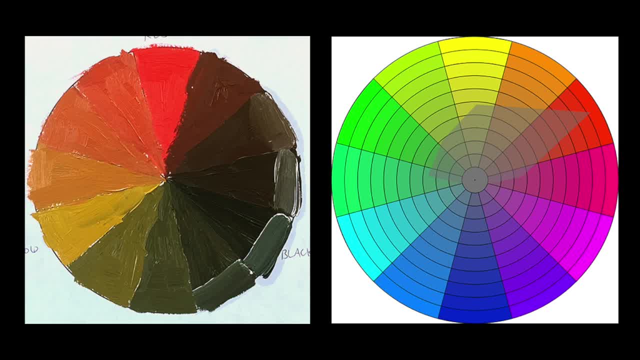 black actually starts looking kind of blue. It's a very interesting visual effect. Another benefit you can see by looking at this color wheel is what a wide range of skin tones you get If you look from your yellow to your red and then going into your black. you've got this. 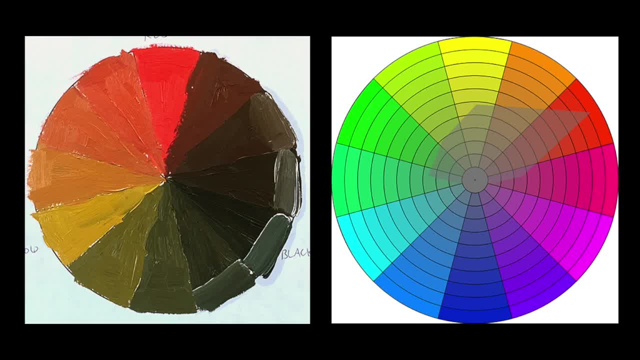 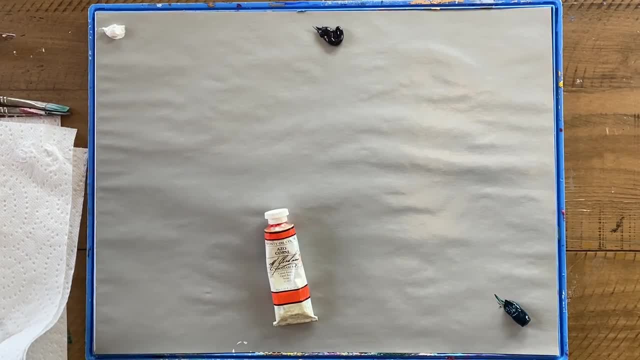 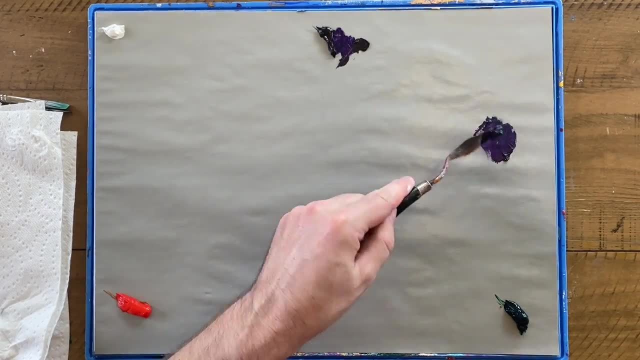 lovely, Expansive, different skin tones to choose from For our fourth set of primary colors. we're going to do something really crazy. We're going to use the three secondary colors as our primaries. What is that even possible? This demonstrates another advantage of limiting your palette. 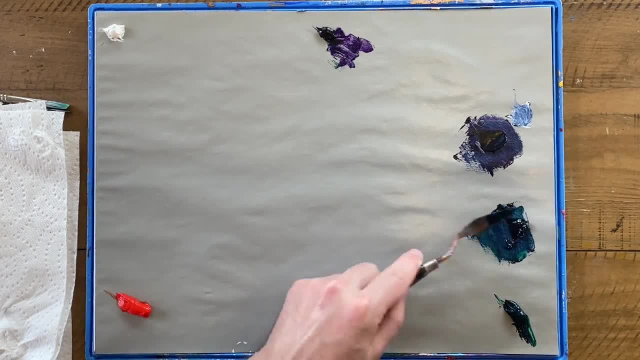 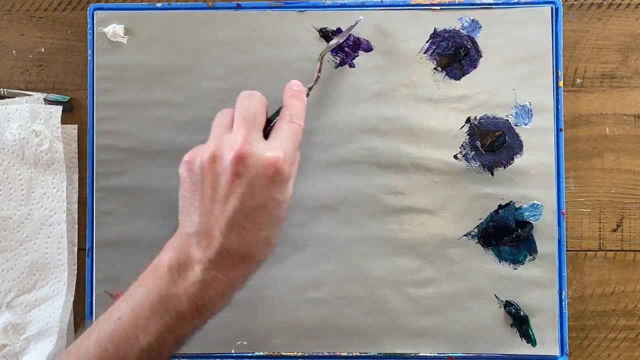 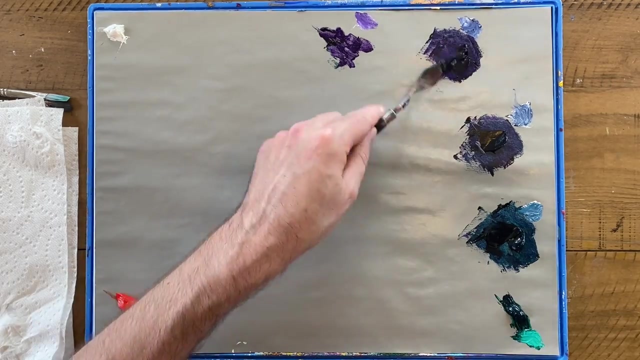 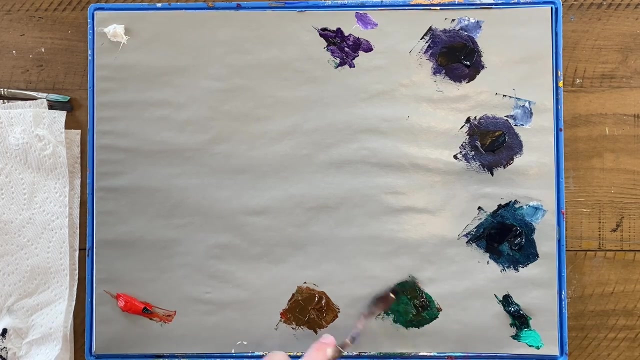 You can use the limitation to create atmosphere. Think of the atmosphere on an evening In your backyard: the sun is setting and it's casting this warm red light across your green grass lawn. Look at the specific color of the green grass. now, If you took a color swatch, that green would look very, very neutral. 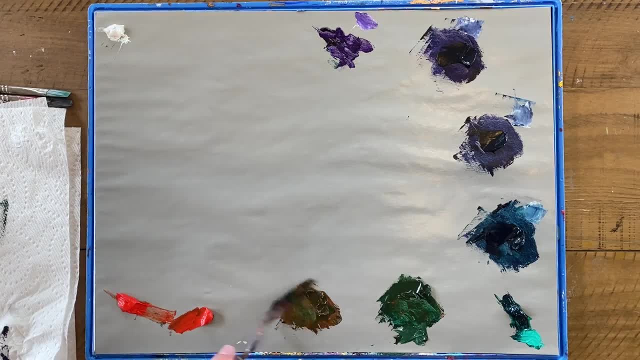 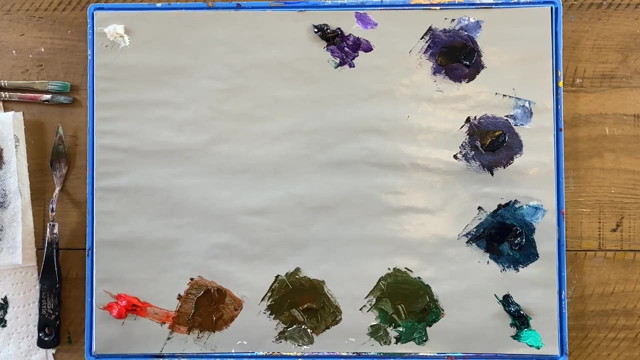 That's because that red light coming from the sun is actually limiting the possibilities of colors that you can see in the world. A truly vibrant green can't even exist under red light. That red light is going to hit the green and it's going to neutralize it way down into 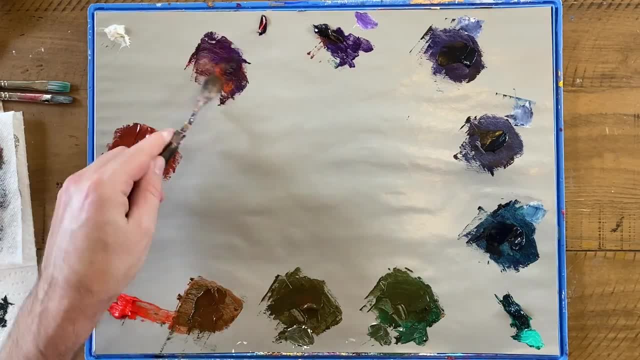 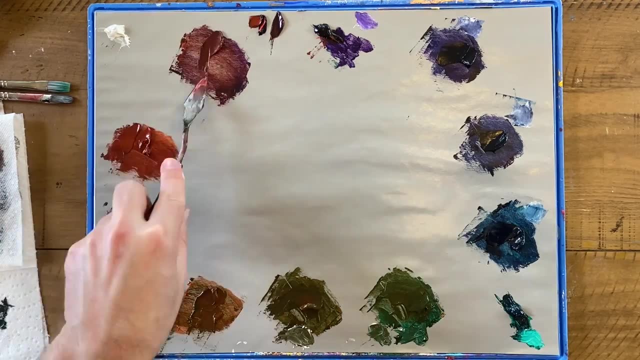 something that is far less saturated. We can use the limited palette to our advantage by creating those similar types of atmosphere. Making a color wheel out of these secondaries will create one kind of atmosphere, but you could literally choose any three colors and make a color wheel. 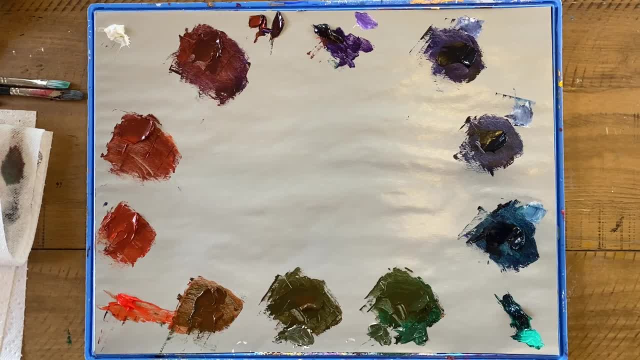 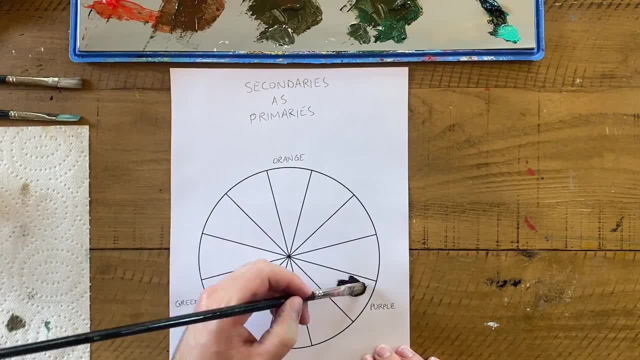 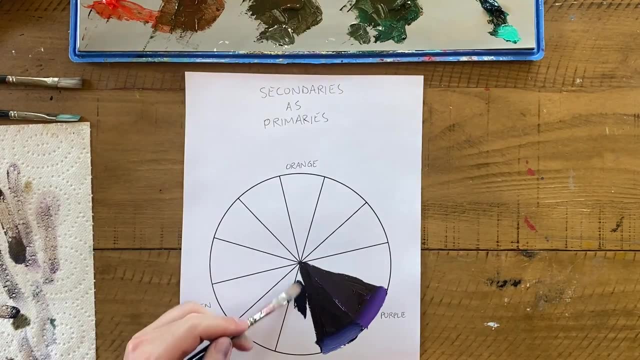 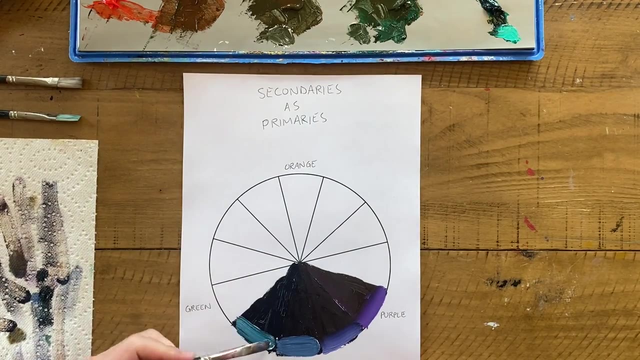 They'll take the entire color wheel and they'll cut out a specific small triangle of colors within that color wheel, which is something called a gamut map. Then the artwork that they create will only include the colors that exist within that tiny triangle of colors. 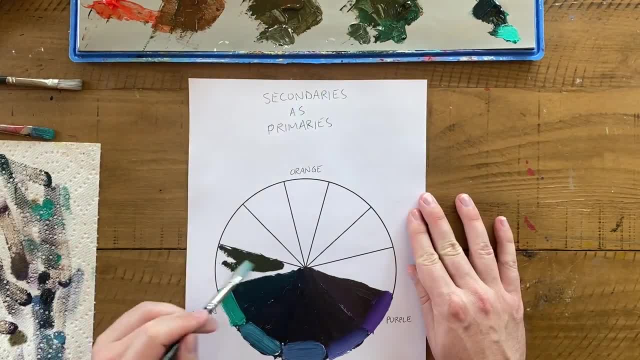 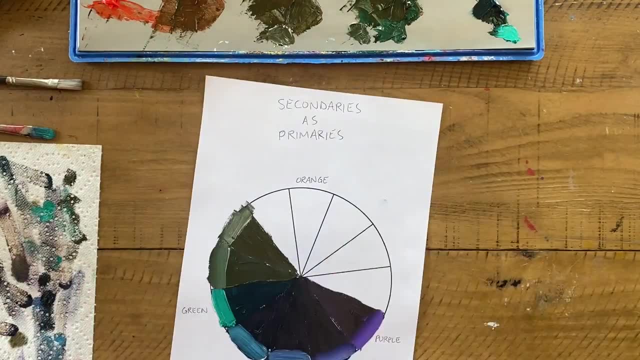 And it doesn't have to be a triangle of colors either. You could make a painting with just two colors. Say, you picked just red and blue and then you mixed a bunch of swatches from there, and then those were the only colors that you could choose for your whole painting. 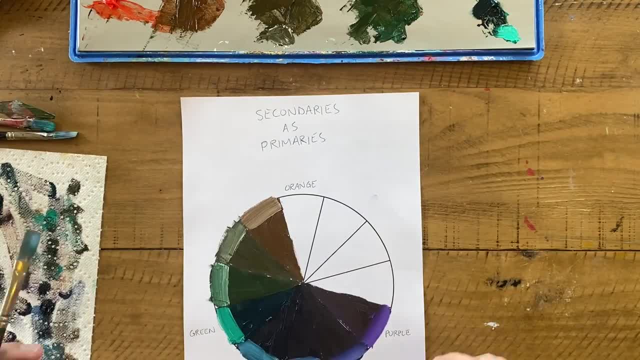 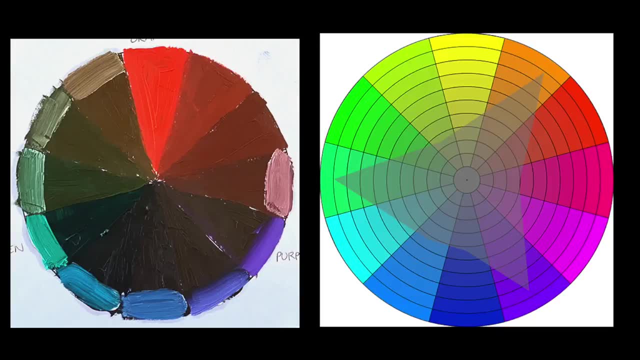 Limiting the gamut of options that you have at your disposal is a fantastic tool for creating a certain atmosphere or visual effect in your painting. All right, so we've got some really fascinating results here. In the past, I never would have thought that I would be able to create a painting with. 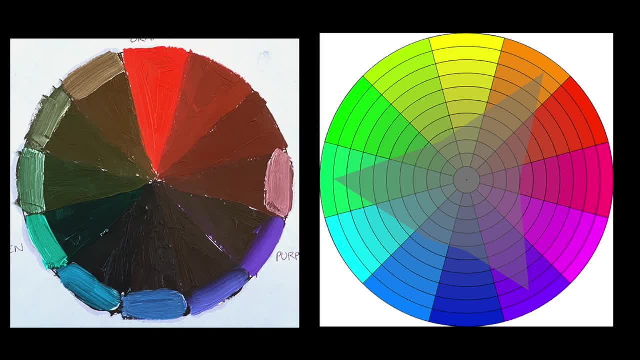 just two colors. I never would have thought that you could take the secondary colors and get primary colors out of mixing them, But that's exactly what we see here. on the palette We've got a really beautiful blue tone that we mixed from purple and green. 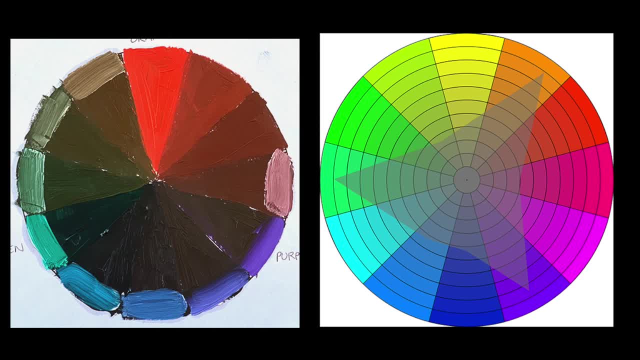 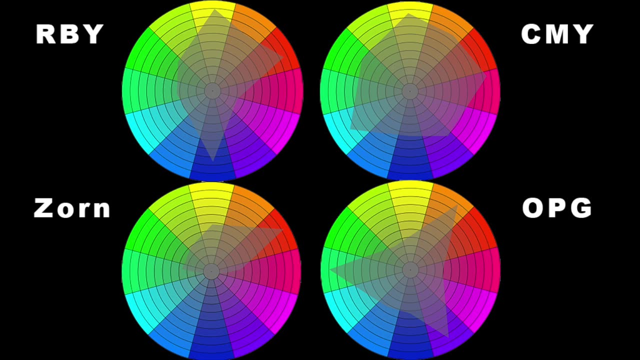 We've got a wonderful brick red that we got out of purple and orange, And we've got a dark brownish yellow that we've mixed from the orange and the green. So our primary colors showdown is complete. And what's the result? Is this like Highlander, where there can be only one set of primaries? 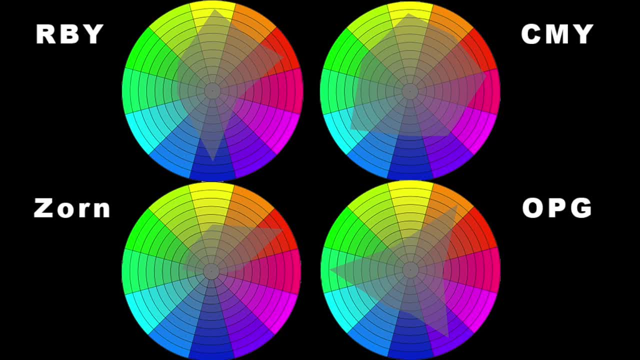 Or is everybody a winner in their own way? Well, I think it's clear from our showdown that there is no one set of primary colors. You can use three different colors to mix an entire color wheel that includes every single hue, Even if it doesn't include every single color. 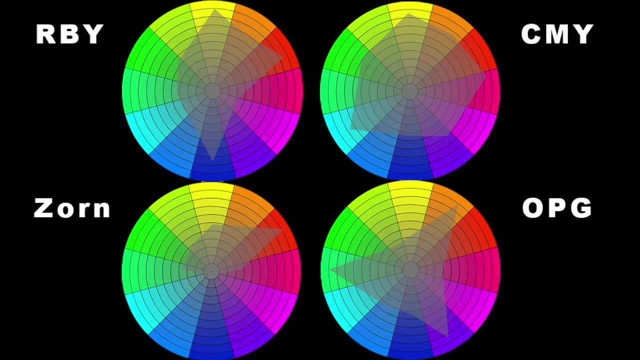 If you're looking for a set of three colors that gives you the widest possible range of colors, I think the winner is clearly the printer's primaries- Cyan, magenta and yellow- But the traditional primary colors of red, blue and yellow are a legitimate choice for. 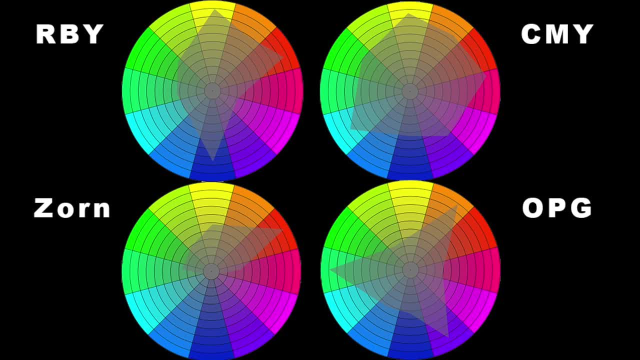 getting a very wide spectrum of color possibilities. One of the reasons the traditional primary colors are so popular is because they're a good combination of colors. The reason the traditional primary palette has lasted as long as it has, I think, is also because we have a good range of pigments that give us paint that has great color, great 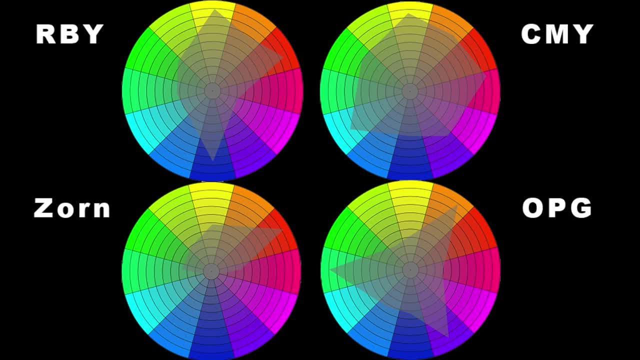 opacity a lot of opportunities for creating the types of paintings we want. You may have noticed in my printer's primaries and in my secondary primaries that the majority of the colors I used were somewhat transparent And some people prefer to paint with more opacity.